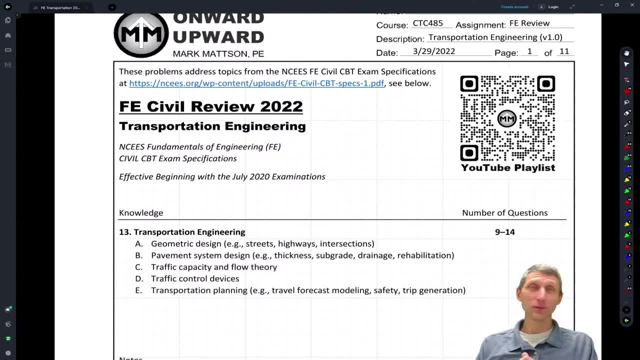 Oh man, what a start to the night, but we'll get going. So, hey, thanks for joining in for the transportation engineering section, the FE review, and we're having a couple audio issues there earlier. I'll try to get those cut out, but hopefully you can hear me well enough. and we 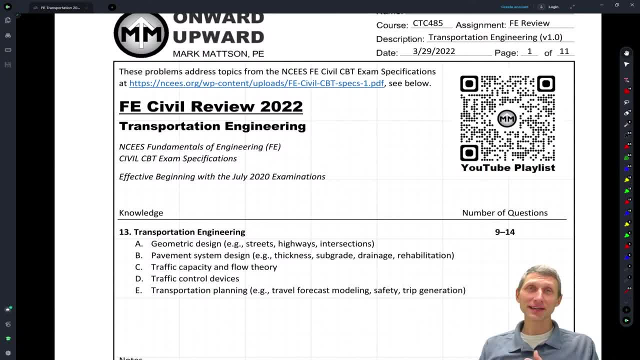 can go from here. So this is the transportation section where there's like a million formulas and like 500 variables, but hopefully we get through a bunch of them And actually the FE review handbook does a good job of sort of paring it down. If you're looking at like the 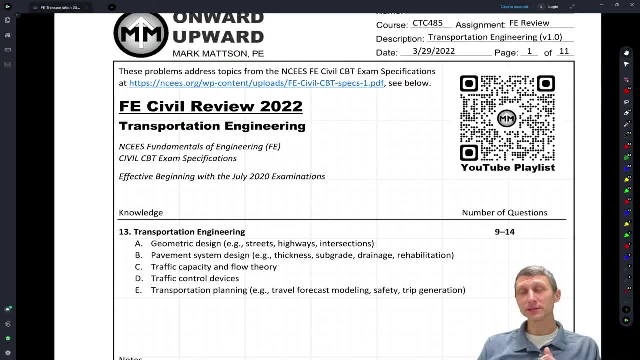 highway capacity manual. that book is just loaded with formulas. So we're going to get into some of those. We're going to hit some with the geometric design. We're going to get hit some with. obviously we have geometric design, pavement systems- I don't hit pavement systems too hard in 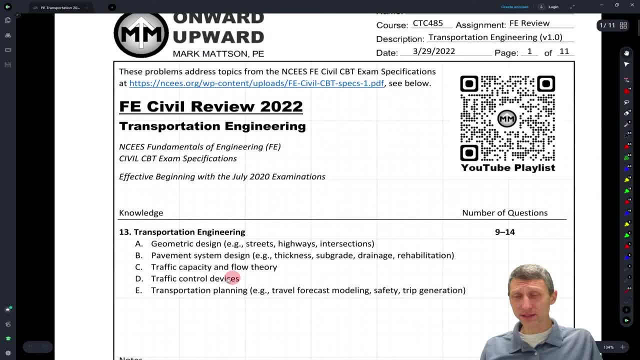 this review Traffic capacity and flow theory. I do get into Traffic control devices. I get into a little bit with timing as well, So we'll see how it goes. Hopefully we can get through all of that and make it through. Okay, So that's the first thing that we're going to look at here for the next couple of weeks. 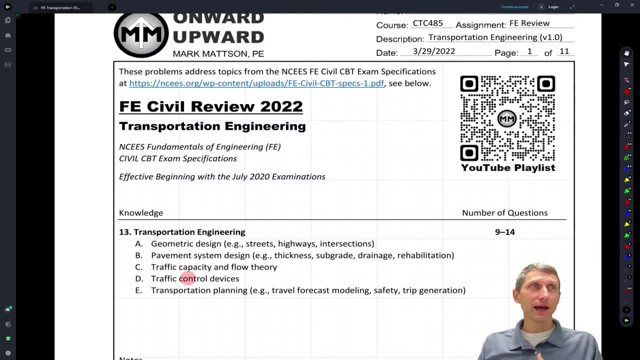 So we're going to hit the gravity model here. We'll talk about the gravity model in a little bit as we go through this. I'll just say that at this point I've learned a couple of things from some people that you know. at one point I think I did a transportation section on this and a past. 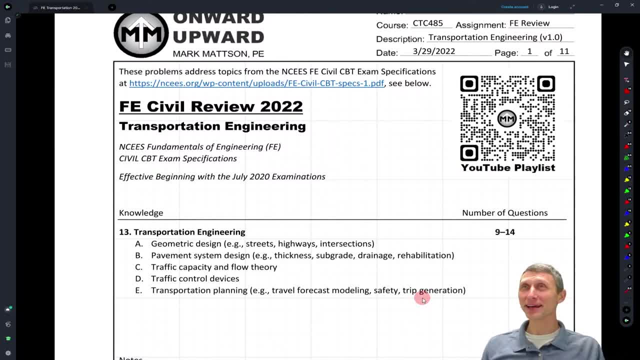 semester And I was like the gravity model that's just like really complicated, So you probably won't get any questions on the gravity model. Well, I had somebody come back and tell me after they took the test. They mentioned that the gravity model is on there, So we are going to hit the We'll jump in and as we get going here, we're going to go to Highway Design, Geometric Design, and we'll get started. So a circular horizontal curve has an angle of 39 degrees between two tangents and a radius. 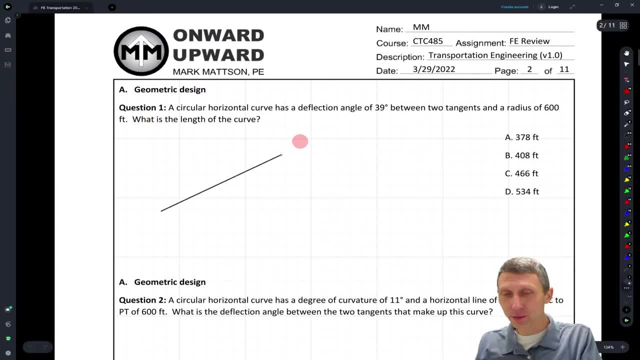 of 600 feet. What's the length of the curve? So basically, what we have here is we're going to start with two lines here- and let me draw that a little bit better, but two lines that are 39 degrees apart. okay. 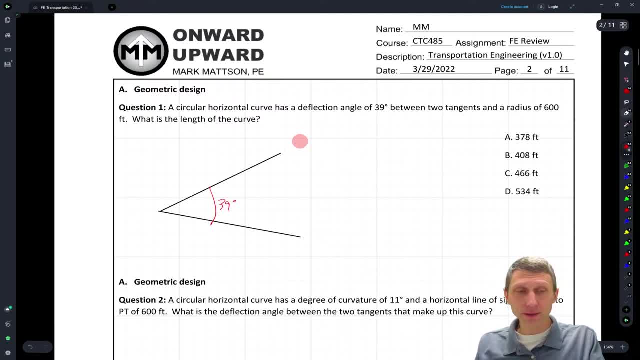 So we got 39 degrees and this is kind of going to be like our road going on here, right. So the question is: we got one tangent coming in, one tangent going out and this curve in between. We know that the radius is going to be 600 feet. so this has a radius of 600 feet and 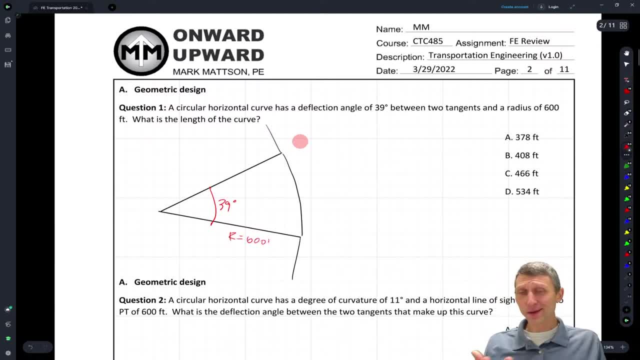 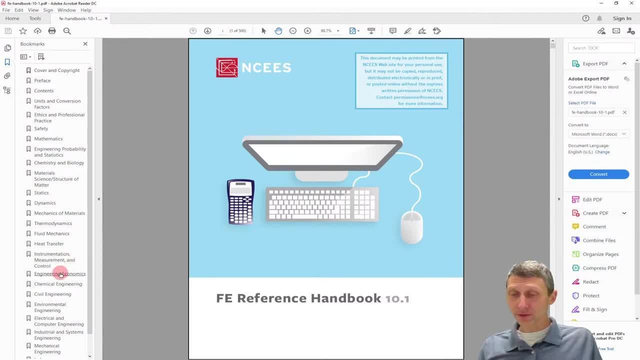 we're just getting warmed up here, so this shouldn't be too crazy. but what we're looking for is the length of the curve. So anytime you get curve questions, the good news is the FE Reference Handbook has a lot of good equations on horizontal curves. 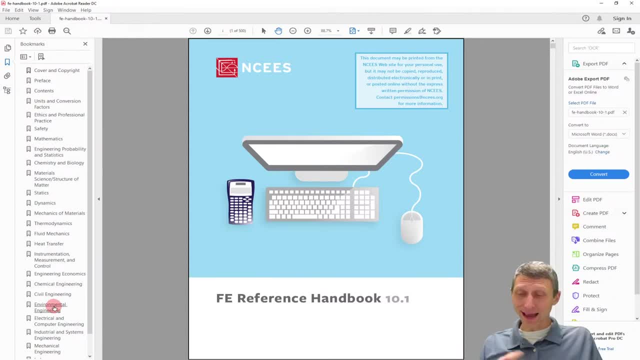 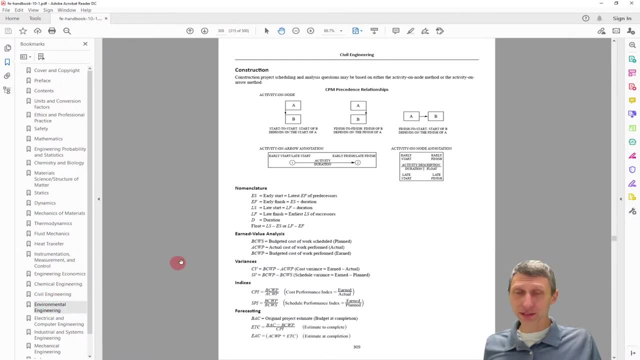 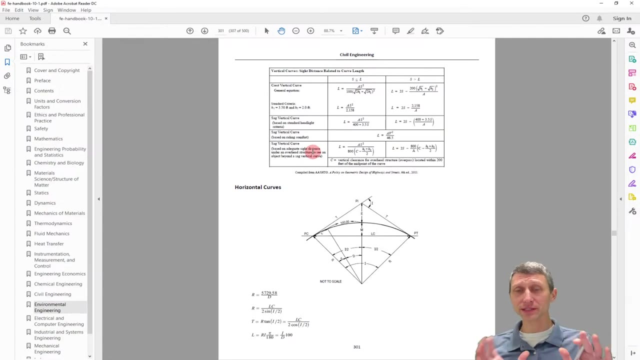 So when I'm going to the transportation section in the handbook, I like to actually start in the environmental section and work my way back, because the transportation section is close to the end of the civil section. So what you see here is there's a section specifically on horizontal curves, right, 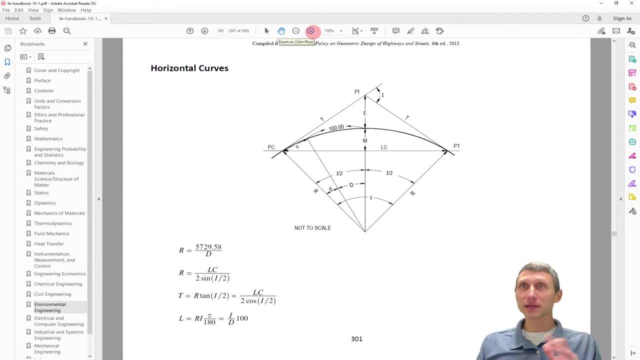 And this is where there is again. there's the transportation. There's a ton of equations, so we have to know those equations, We have to be able to use those equations, figure out those equations and come up with something that works. 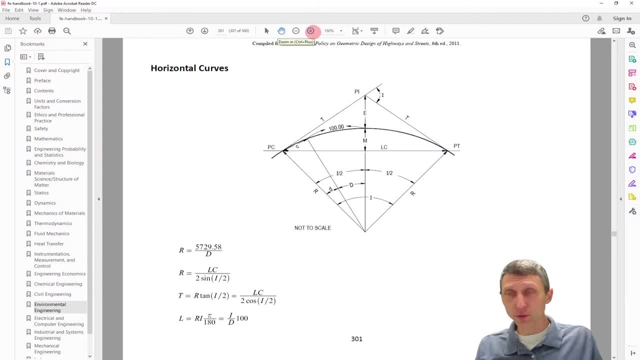 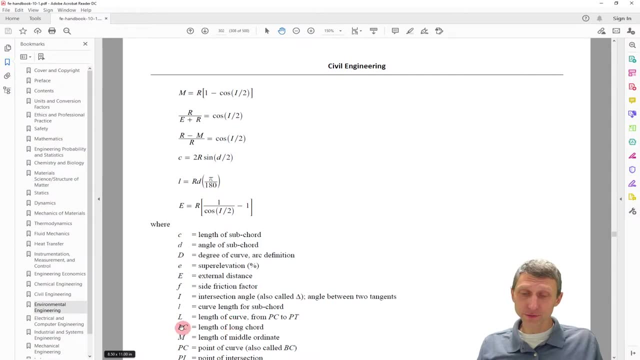 So what we're told here is: we want a length of a curve. so what we're going to do is we're going to look, We're going to see what we can find here, and we see that L is the length of the curve. 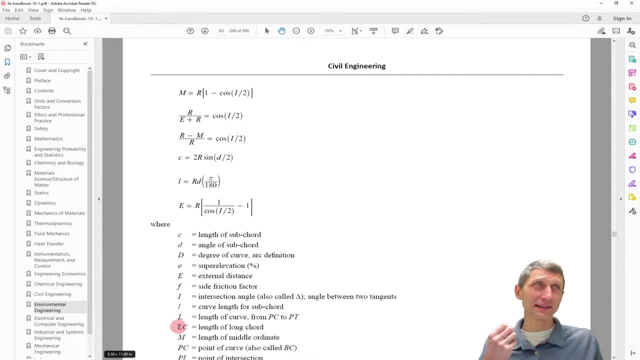 and just I threw this one in there so that you can see L is different than LC, right? LC is going to be The chord length, which is different, So we will use that equation here and keep going. So sorry, I'm still getting set up here. 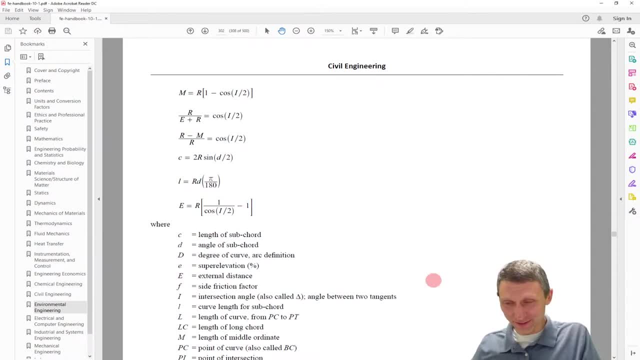 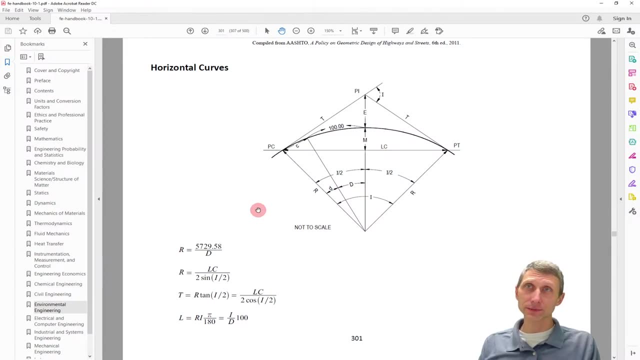 The little hiccup in the beginning made it a little bit of a challenge, but what we see here is we're looking for an equation with L, and a lot of times that's what you're going to be doing when you're getting into some of these horizontal curve questions is 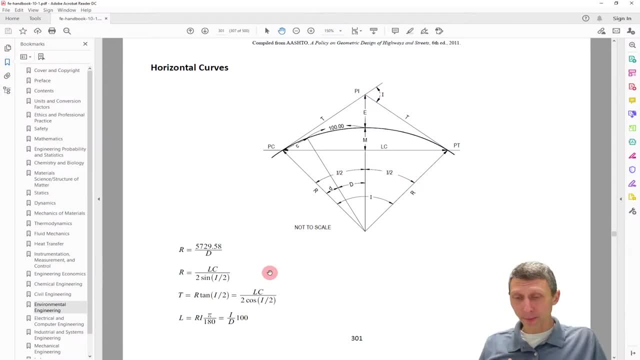 what equation works right, What do I have, What do I need to know And what will work here? So I know I have L and here's the equation for L, right, And the equation basically starts with R, the radius, the deflection angle and a conversion. 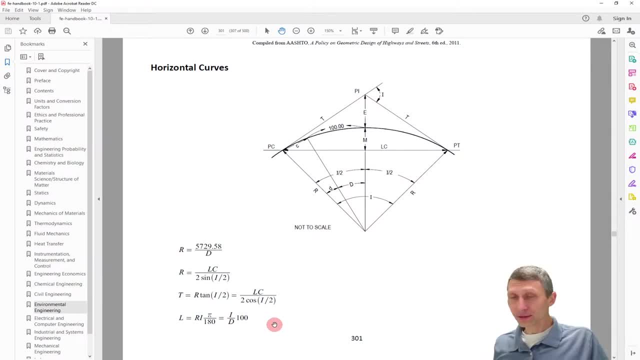 from degrees to radians. So this one is honestly, about as easy as you could hope for, and they probably won't be this easy, but if they are, that's okay. We'll take the easy ones along with the hard ones, but what we have here is a length of 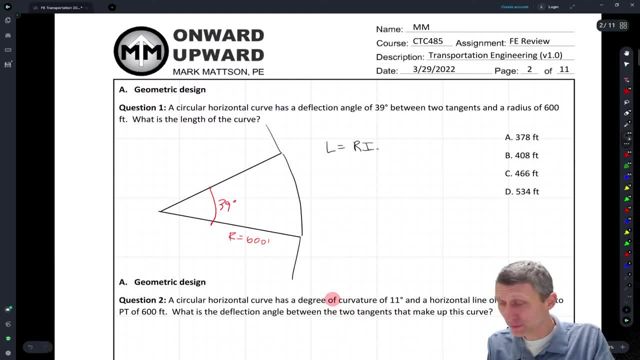 curve equals RI times pi over 180 degrees. okay, So we basically have what we need here and we're just going to plug in, right. So 600 feet times I, which is that deflection angle of 39 degrees, and we're going to convert. 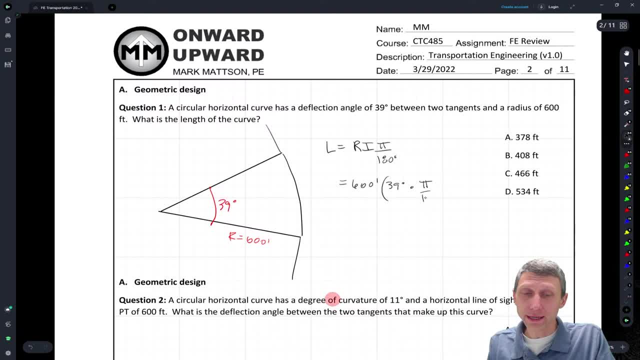 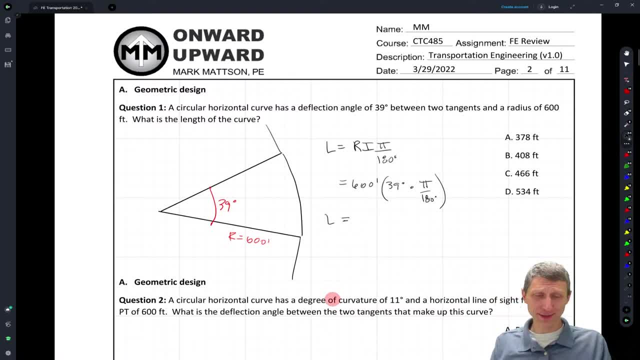 Well, I think I'm going to put that one in here, but hopefully I didn't screw that one up. but 600 times, 39 times pi over 180 is just going to be. you got to love the 130 pi and the TI-36X, but you know how you get the. there's right above the enter button. 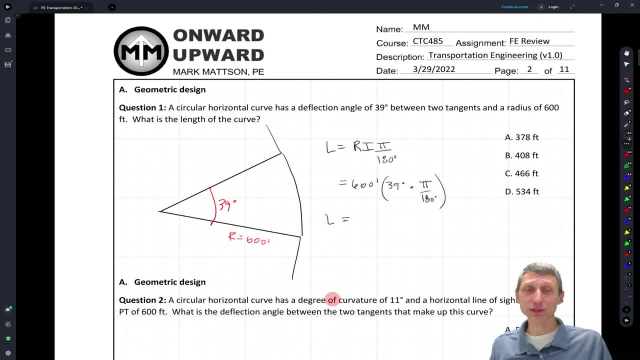 there's that little arrow button that takes it out of pi and into actual feet. So that's going to be 408 feet and we're off to the races. okay, So some of these questions are going to be easy. Some of them are going to be a little bit more complicated, right? 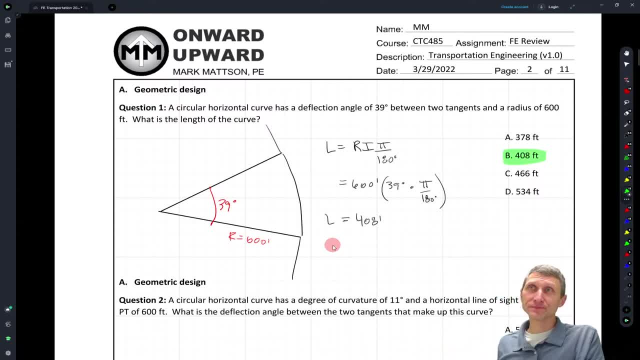 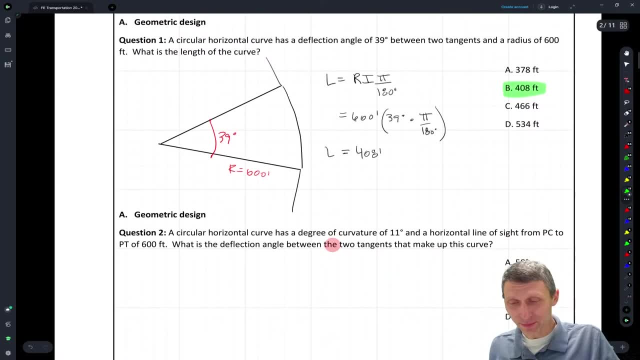 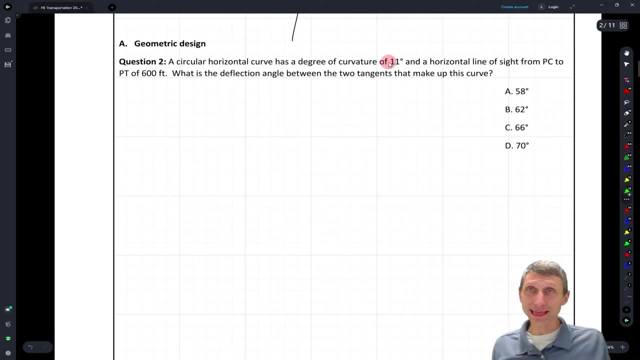 But when you get into curves you do have to know your terminology. You have to know how to make each of these work. So we'll just keep going. So question two: right, Horizontal again, we have a circular horizontal curve, degree of curvature of 11.. 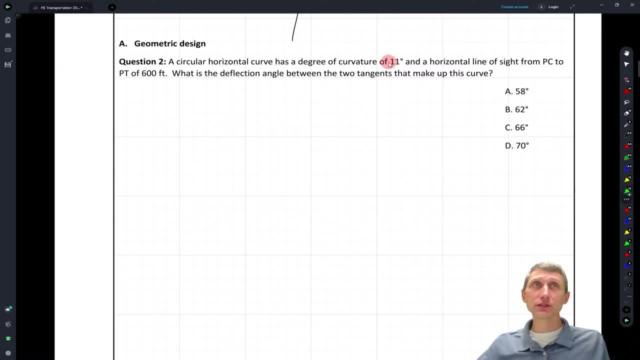 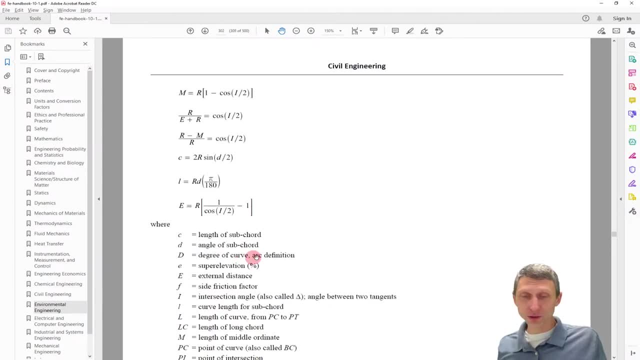 So degree of curvature is different than that deflection angle. The degree of curvature is basically how much curve you have per 100 feet. So the degree of curve is how much curve you have per 100 feet. So in this case it's going to be 11 degrees per 100 feet and that's where we're going to start. 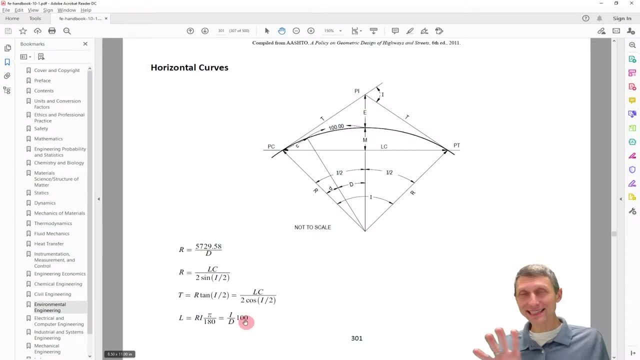 And you might say: well, how do you know that? It kind of gets into this equation down here too? So the ID over 100, that's that where we go from I to D, it's we get that 100 in there. 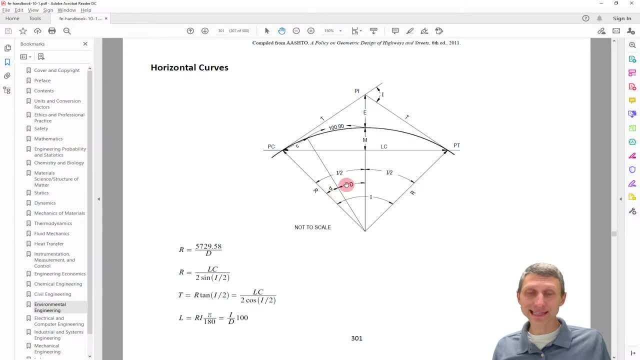 and that's what we're doing, And even you can see it. you can see it here, right? This D is that deflection, or the degree of curve which is per 100 foot of arc length. OK, so where are we going with that? 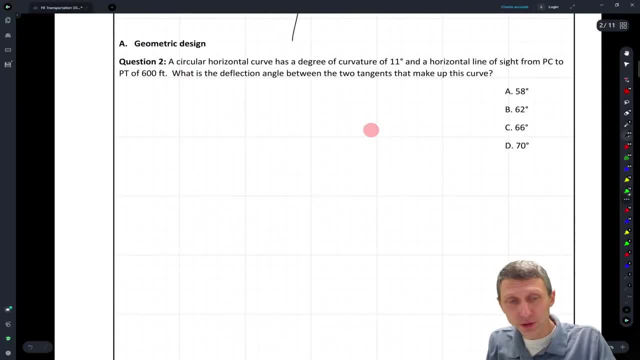 Well, first, that was just what we're given. So we know that we have a curve here, right, And you know let's draw on our curve again, Right. So we're going to draw on some curve, but we're not told the total angle. 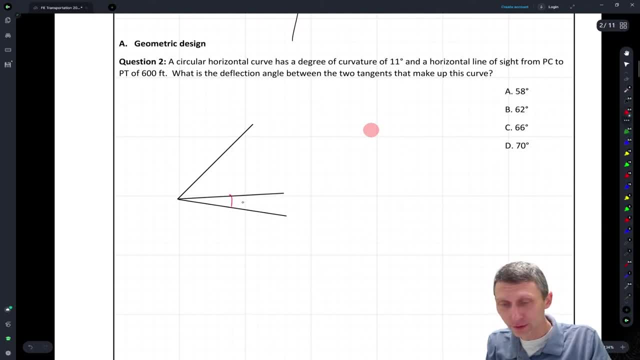 We're just told this deflection angle, We're just told the total angle of you know what, 11 degrees per 100 feet. So we got a tangent coming out here, a tangent coming in here, and we have this curve, that kind of goes. 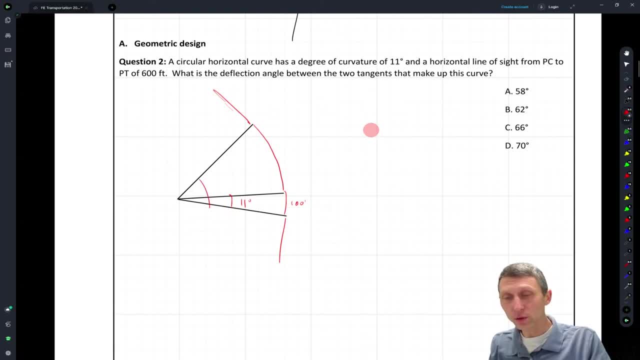 And the question is asking: you know what's the deflection angle, this total angle that makes up the curve right? We do know that we have a horizontal line of sight from the PC to the PT. So some more language here. 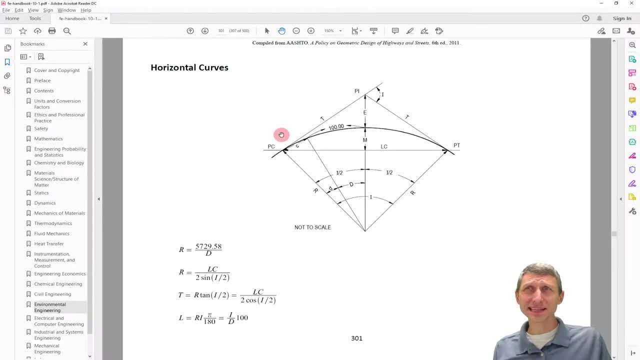 But what we want to do is come back to our diagram And we see the PC is the point of the curve. So the start point, the PT, is where it goes back to tangent right. So this is: this is a tangent line that goes straight out and that's going to be, that's going to be the roadway, that's no longer the curve. 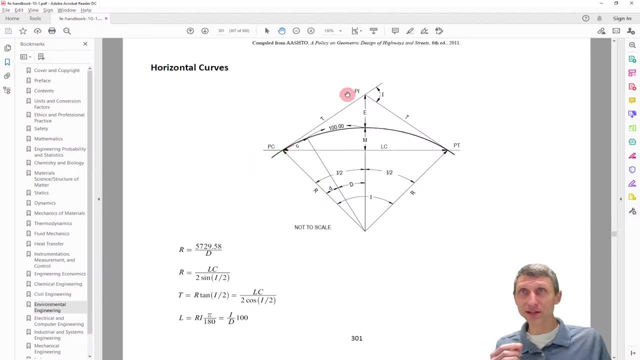 So the PC is the beginning, the PI is the point of intersection. the intersection, if you extended the two tangents all the way out. So what we're given, though, is we're given the point of curve, the distance that you can see straight from the point of curve to the point of tangent. 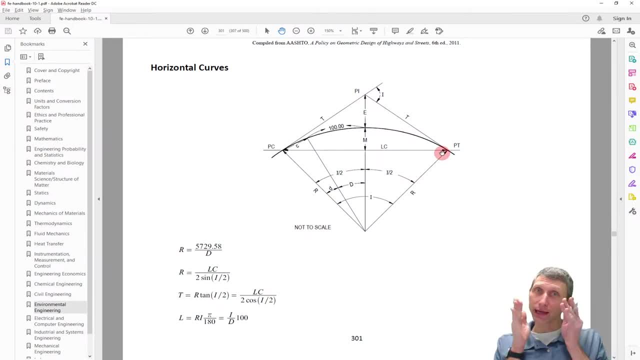 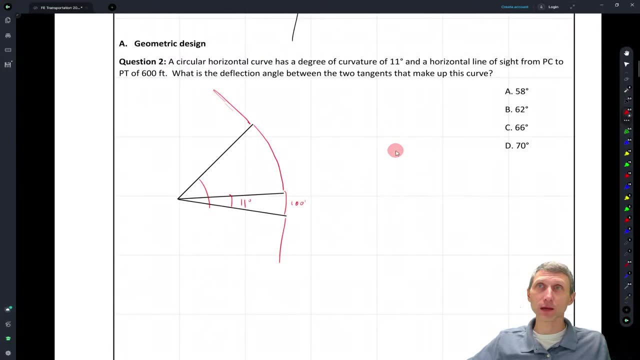 And the last time I looked I didn't look around a curve, I had to look straight, Right. So the idea here is that's the, that's the LC value, And I didn't say that's LC, I didn't say it's the, the chord length you know. and that's where it does help to also kind of understand here that some of these, some of these terms aren't going to be defined exactly the way they are in the handbook. 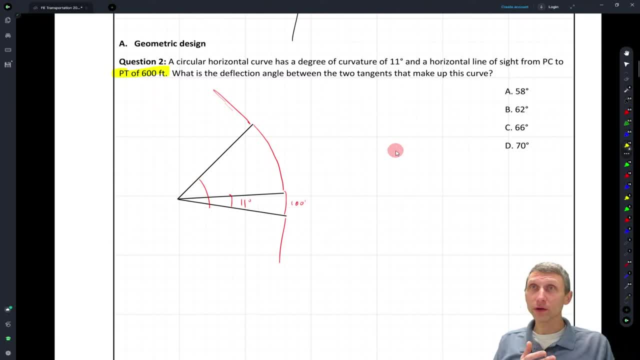 But you can still make them work. So so, let's see, Let's keep going here. So So, let's come back to our equations. but but actually, before we come back to our equations, what we have here is is: LC equals 600 feet. 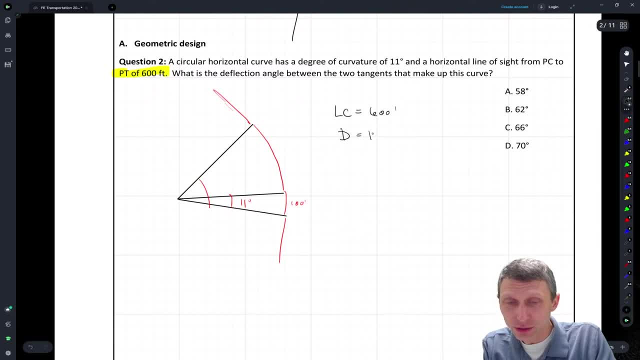 OK, that's the chord length. We have this degree of curvature of 11 degrees. OK, so what we're trying to find is this deflection angle, and that's that's what we're going to do. So let's come back to where we, where we are here. 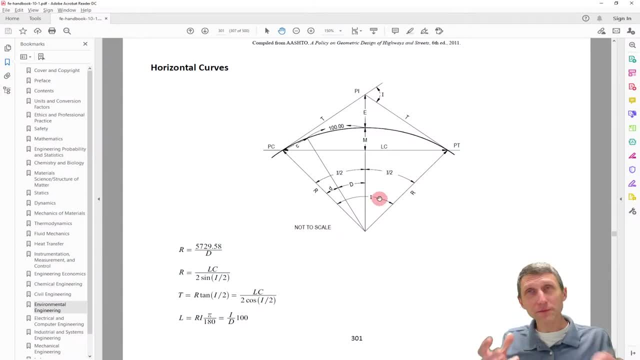 That deflection angle is this: I Right. So we're looking for Something that relates I to D, to LC, and what we can see here is we do have kind of this equation that we've LC and I, but that doesn't give us D. 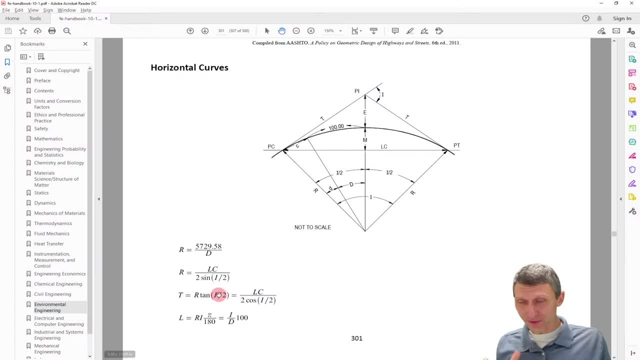 But then what else do we have? We have, you know, we have a couple of things going on. We do have a radius here that that will relate us. So this becomes kind of a two step curve problem. So we have to find- I 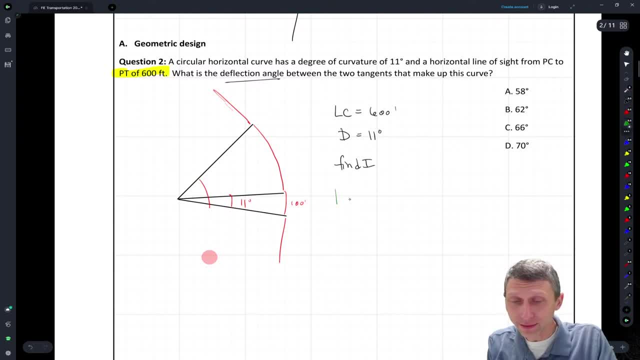 Right, We have to find I, But first, Before that we can do that, Let's first find the radius. I'll tell you why in a minute, But first we're going to use that radius formula is equal to: so the radius equals five, seven, two nine point five eight right divided by D. 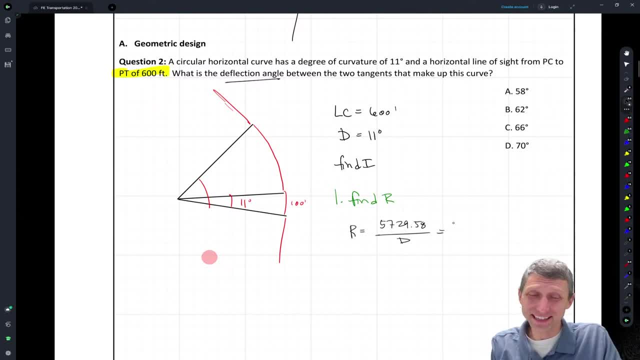 That's the formula in. this is a conversion, It's, it's, it's a conversion. OK, so we could go and derive it, but you don't need to, So let's just do this. So we're going to take this out, divide it by our eleven degrees, and it's going to give us five hundred twenty one feet. 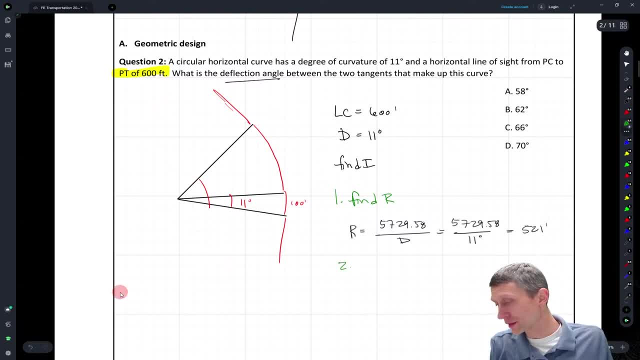 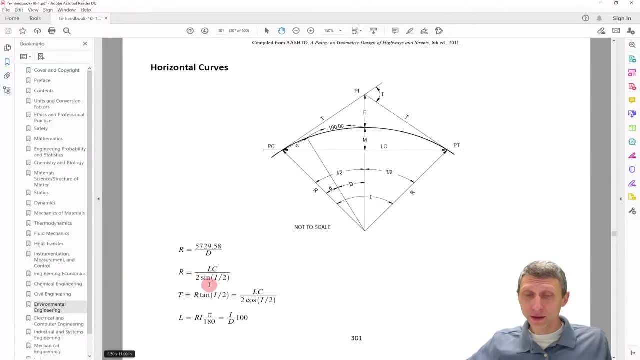 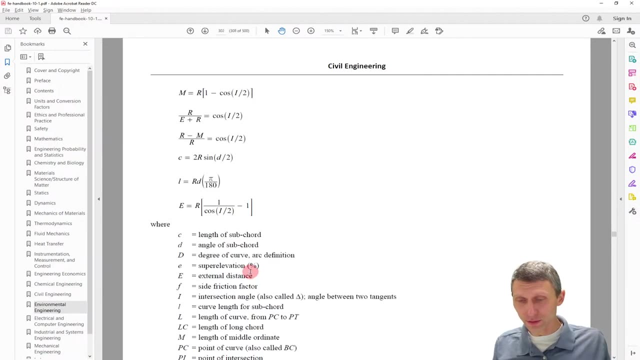 OK, and then let's go to step two here, and step two, we're going to say: we're going to use another equation: So now that we have our, we can come back and we can say: now we have our, we're going to have LC to sign, I over two and one thing just to let's. let's take a look at this for a second. 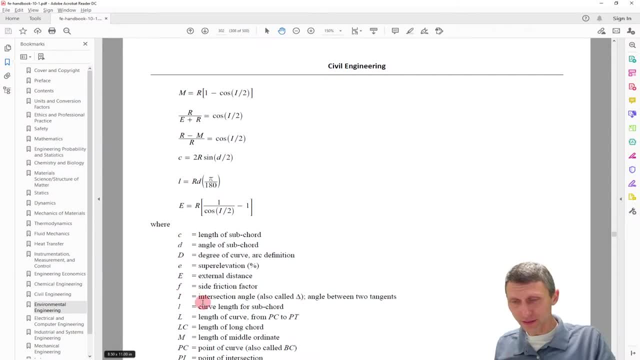 But I was just curious if this told us whether our, our our angles are in degrees or not. and it doesn't, But that's typically what happens, And if we need radians, we'll. we'll come back to radians, So let's come back here. 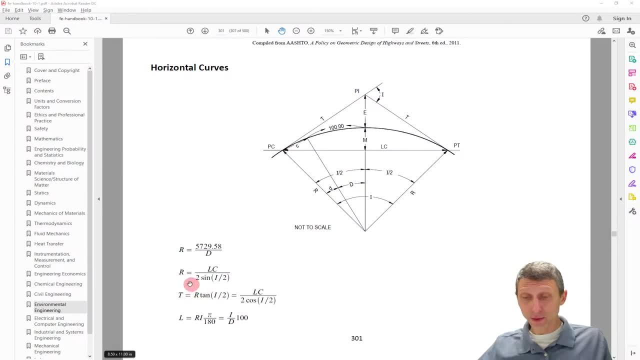 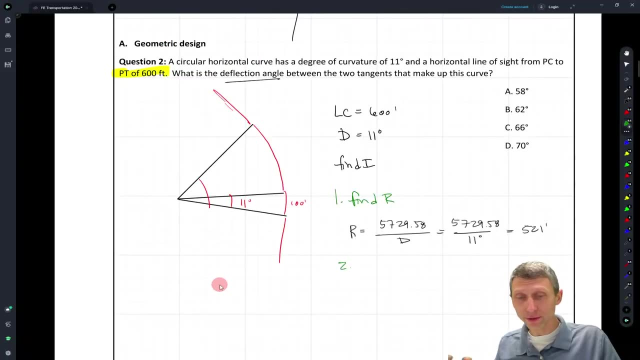 But we do know that this formula here, now that we have our, we can and we have LC, now we can solve for I. OK, so let's come back here. We'll use that formula. So our second thing that we're going to do here is we're going to find: I.